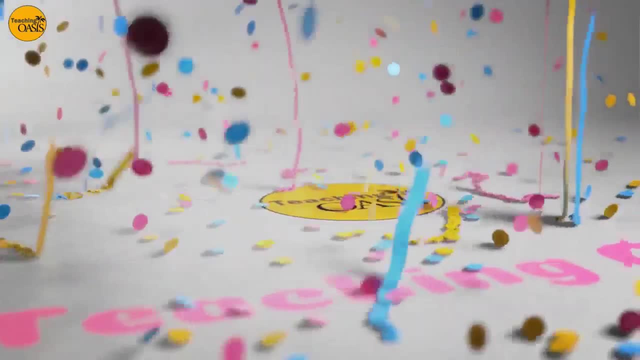 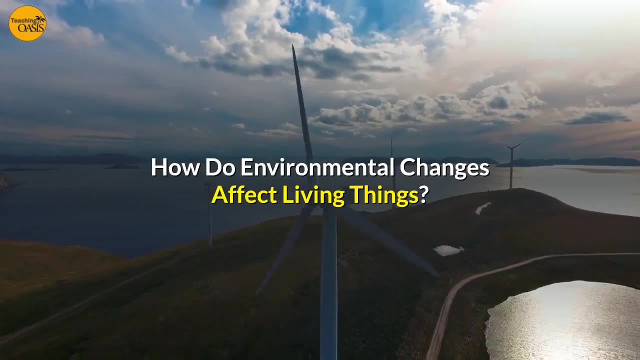 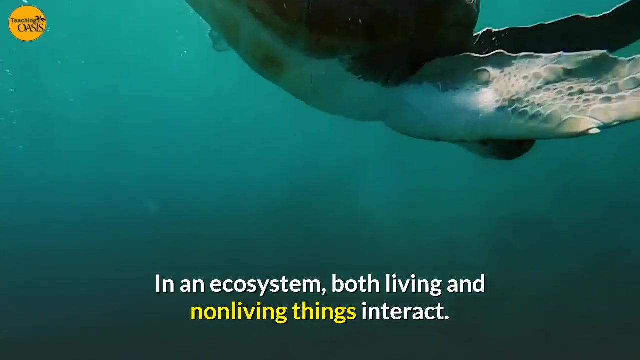 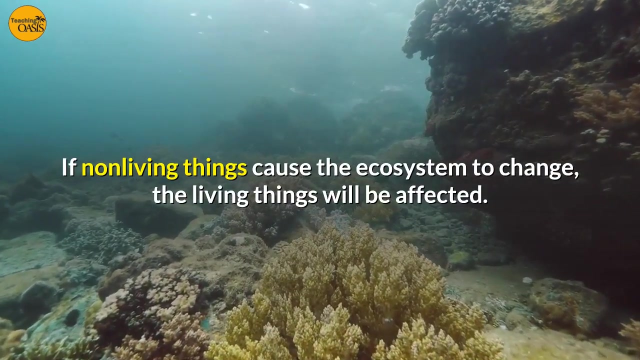 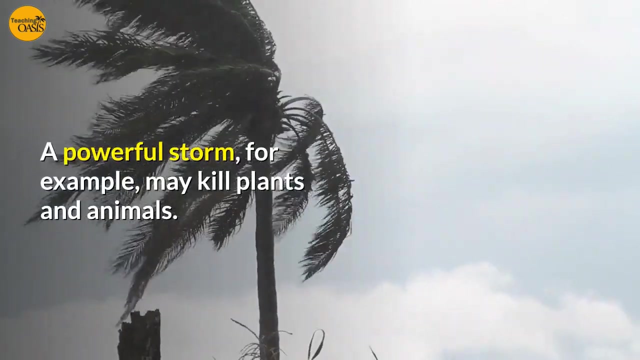 How do environmental changes affect living things? Fragile ecosystems. In an ecosystem, both living and non-living things interact. If non-living things cause the ecosystem to change, the living things will be affected. A powerful storm, for example, may kill plants and animals. 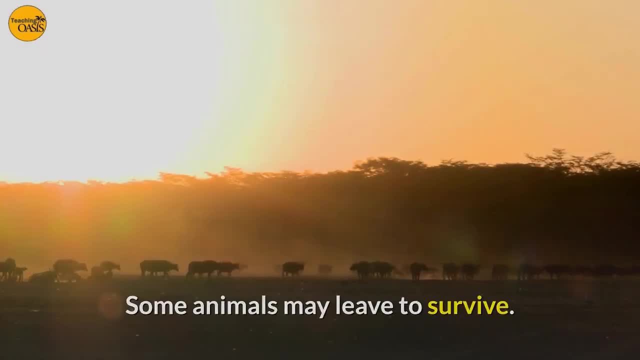 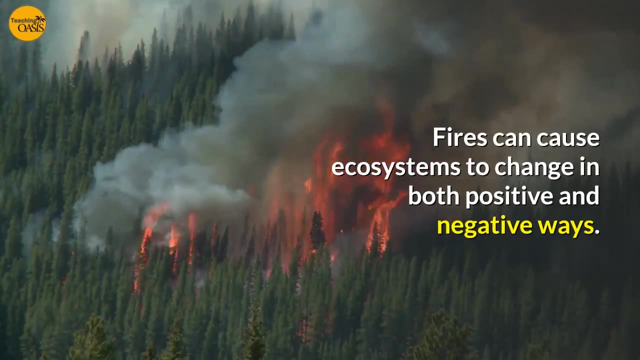 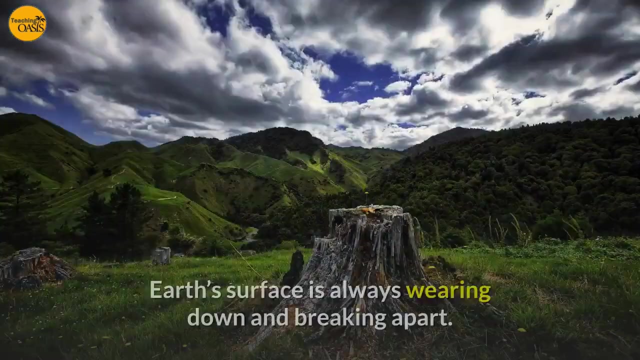 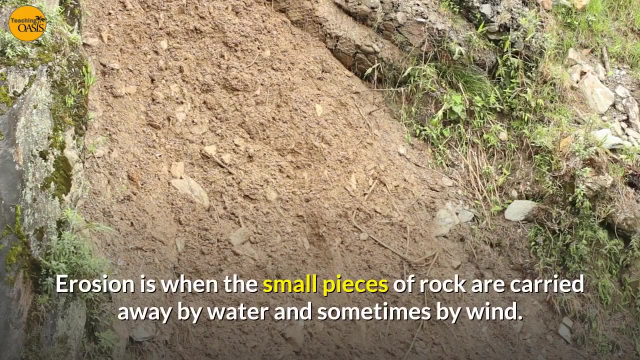 Some animals may leave to survive, Others may stay and compete for resources. Fires can cause ecosystems to change in both positive and negative ways. The right amount of water. Earth's surface is always wearing down and breaking apart. Erosion is when the small pieces of rock are carried away by water and sometimes by wind. 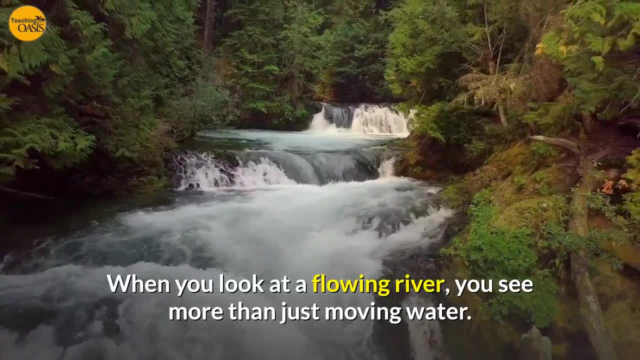 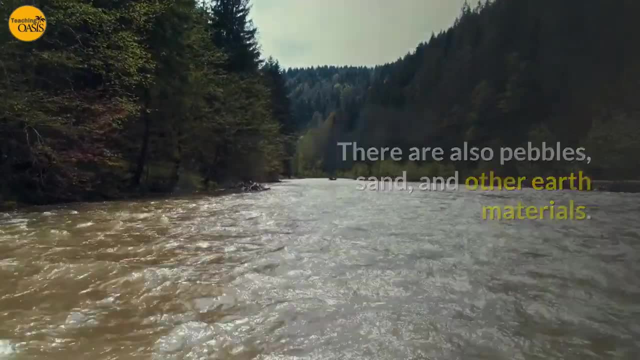 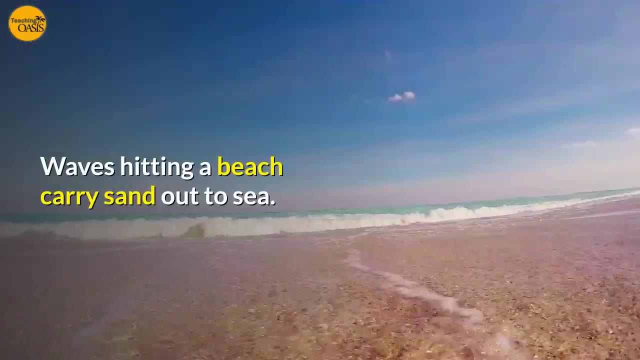 When you look at a flowing river, you see more than just moving water. There are also pebbles, sand and other earth materials. This is erosion. Ocean waves can also cause erosion. Waves hitting a beach carry sand out to sea. 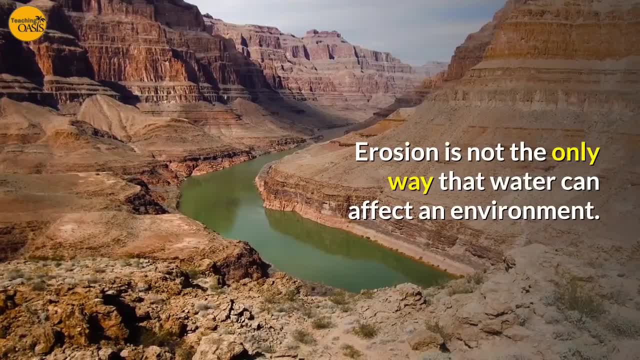 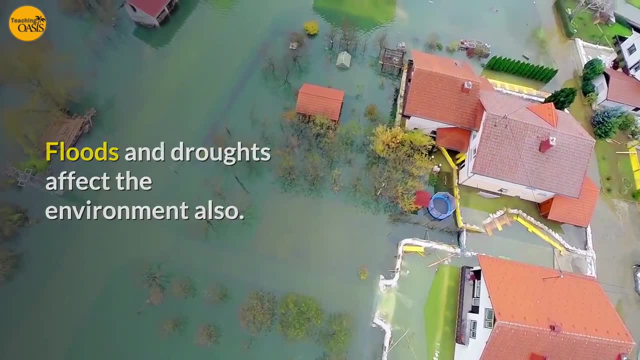 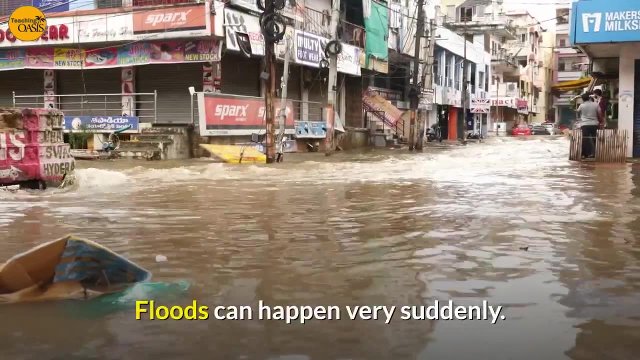 Erosion is not the only way that water can affect an environment. Floods and droughts affect the environment also. A flood is a large amount of water that covers normally dry land. Floods can happen very suddenly. A drought occurs when it does not rain for a long time. 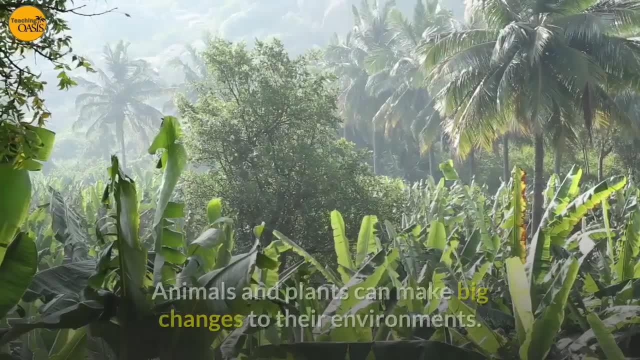 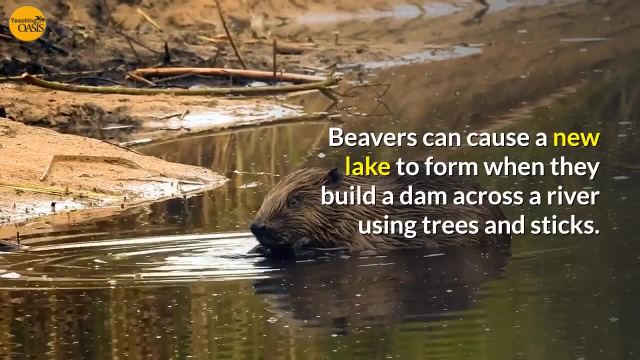 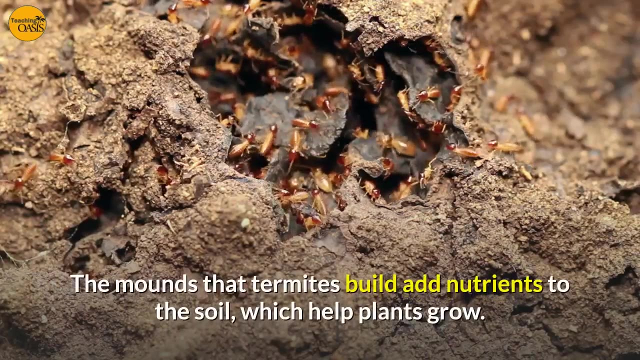 Natural changes. Animals and plants can make big changes. Beavers can cause a new lake to form when they build a dam across a river using trees and sticks. The mounds that termites build add nutrients to the soil, which help plants grow. 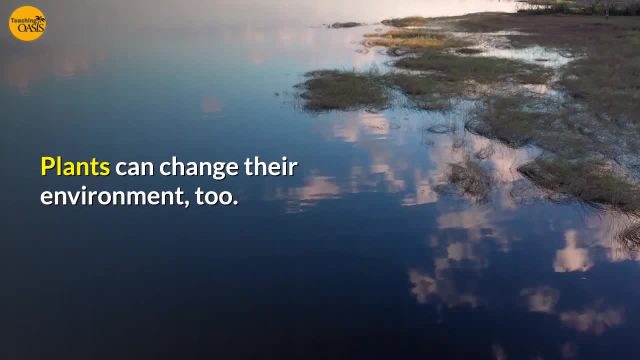 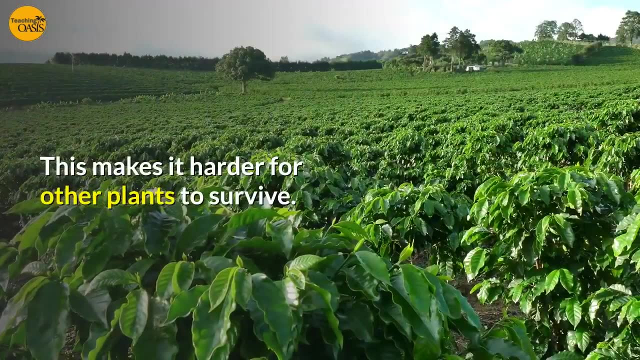 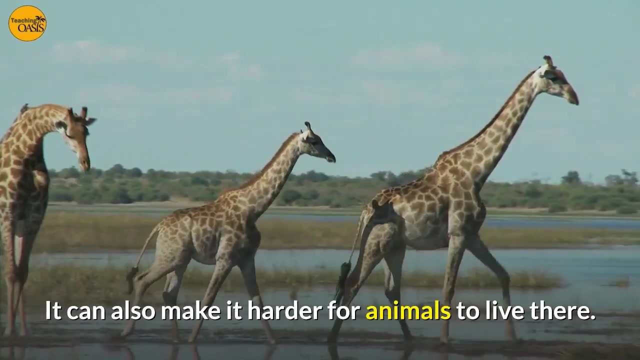 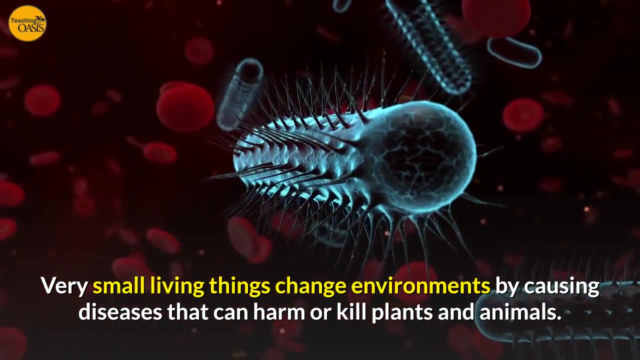 Plants can change their environment too. One kind of plant may take over all the space in an area. This makes it harder for other plants to survive. It can also make it harder for animals to live there. Very small living things change environments by causing diseases that can harm or kill plants and animals.